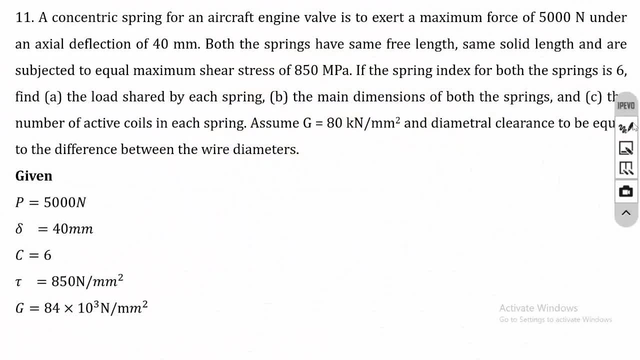 In the previous lecture we have seen the basic concepts of concentric spring and how to find the load shared by each spring. In this lecture we are going to solve a problem on that. A concentric spring for an aircraft engine valve is to exert a maximum force of. 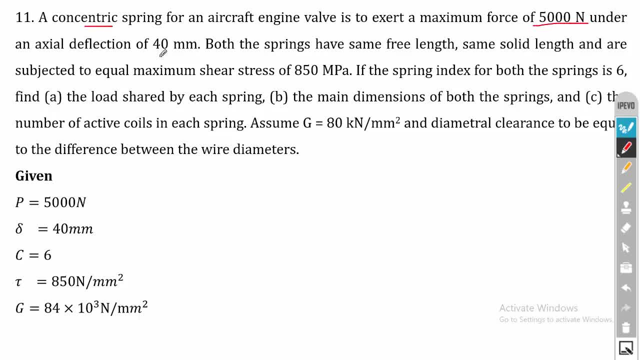 5000 N under an axial deflection of 40 mm. The load is given as 5000 N, That is load carried by the concentric spring. It is common for both inner and outer spring. The deflection del is 40 mm. Both the springs have same free length, which means LF1 is equal to LF2.. 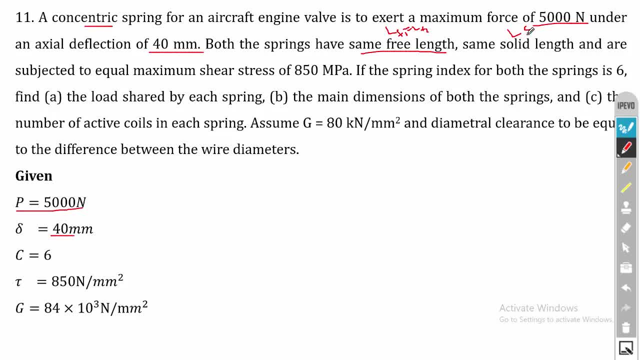 Same solid length, LF1 is equal to LF2 and are subjected to equal maximum shear stress of 850 MPa. So here the tau1 is equal to tau2, because we know that in concentric spring both the springs are made of same material. So tau is equal to 850 MPa. That is common. 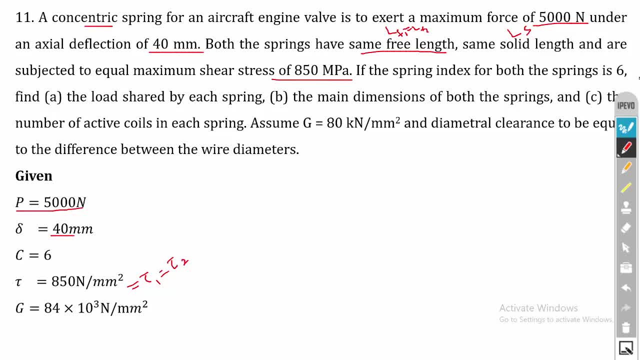 for both inner and outer spring. The spring index for both inner and outer spring is equal to tau1.. So tau1 is equal to 850 MPa. That is common for both inner and outer spring. The spring index for both the springs is equal to 6.. So for concentric spring, always the spring index is same and 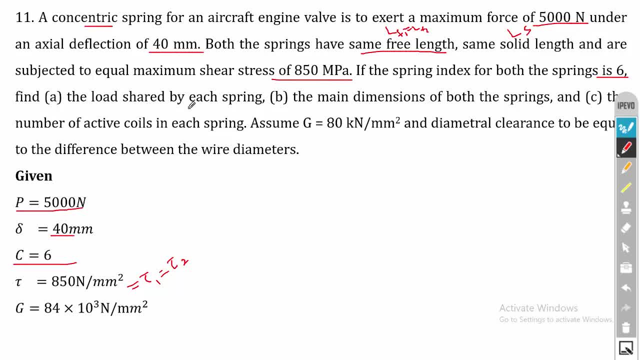 it is 6.. Find the load shared by each spring, So that is P1 and P2.. The main dimensions of both the spring, that is wire diameter and coil diameter, So both for outer spring and for inner spring. The number of active coils in each spring, So small: n, n1 and n2.. Assume G is equal to. 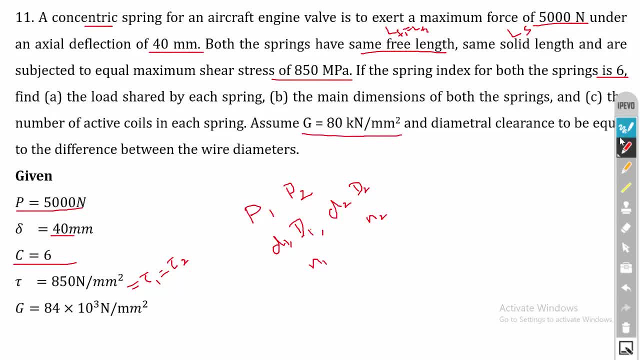 80 kN per mm2 and diametral clearance to be equal to the difference between the wire diameter. So the meaning for this statement is: in the previous lecture we have seen that P1 by P2 is equal to C divided by C-2- the whole square. So that is the reason. that is the meaning. 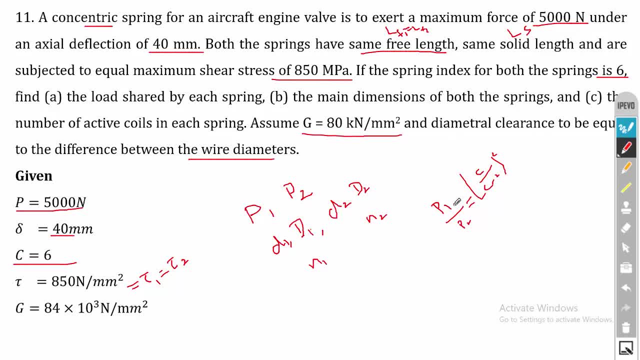 for this line. Anyway, if it is not given. also, we have to take P1 by: P2 is equal to C by C-2, the whole square. So remember that in the derivation I have considered the 1 as outer spring and the 2 as inner spring. So P1 means load acting on the outer spring. 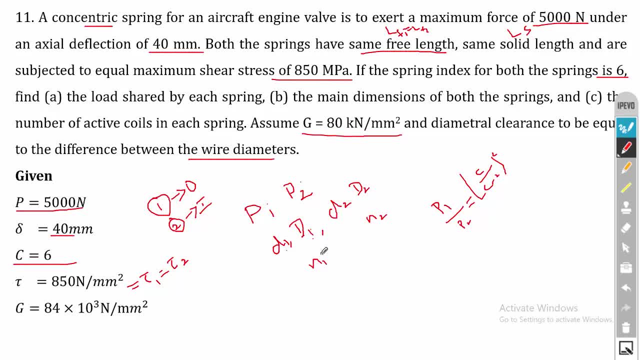 and P2 means load acting on inner spring. Similarly, D1 and D2 for outer spring. I mean D1 and capital D1 for outer spring, Small d2 and capital D2 for inner spring. N1 is the number of turns of the outer spring. 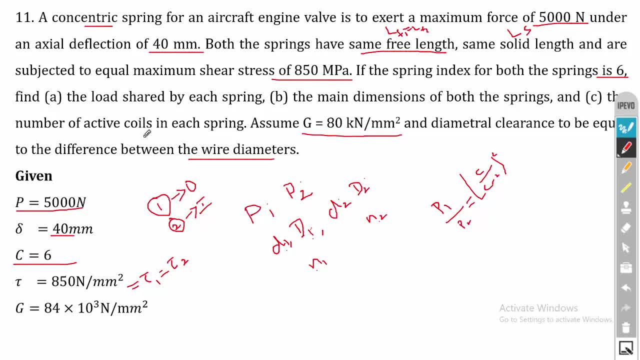 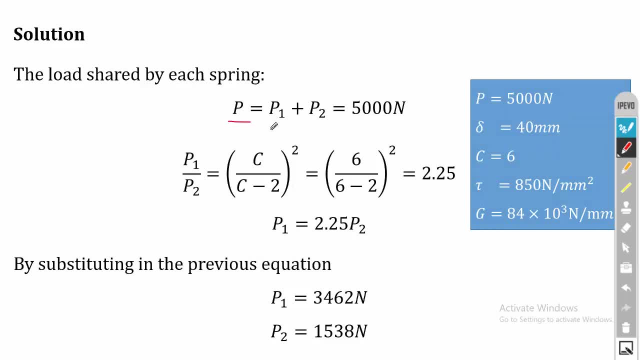 and N2 is the number of turns of the inner spring. So first we will start with the load shared by each spring. You know that capital P, the total load, is equal to summation of P1 plus P2, that is, load acting on spring 1 plus load acting on spring 2, that is equal. 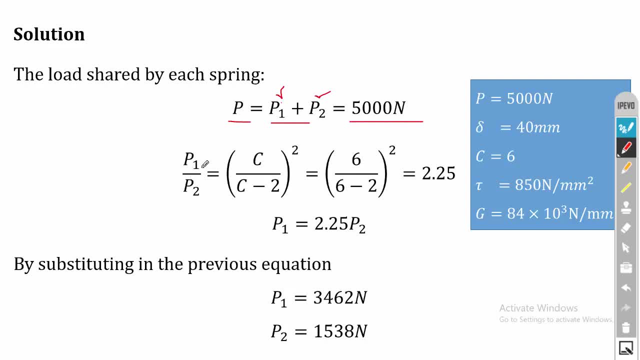 to 5000 Newton. Further, the relation between the load is: P1 by P2 is equal to. so actually we have two relations. So one is the summation of P1 and P2 is equal to P. The second one is P1 by P2 is equal to C divided by C-2, the whole square. 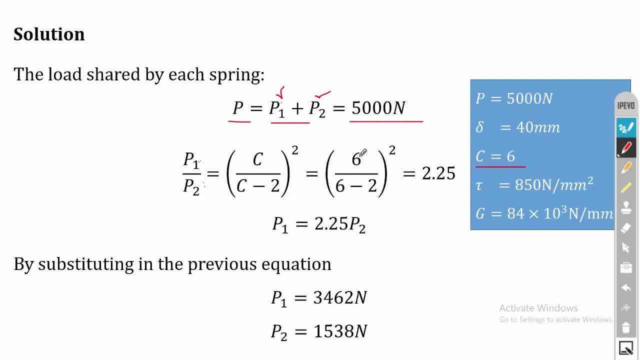 And in the problem the C value is given as 6, so we can substitute it. It is 6 divided by 6-2, the whole square that is equal to 2.25.. So further P1 is equal to 2.25 times of P2.. 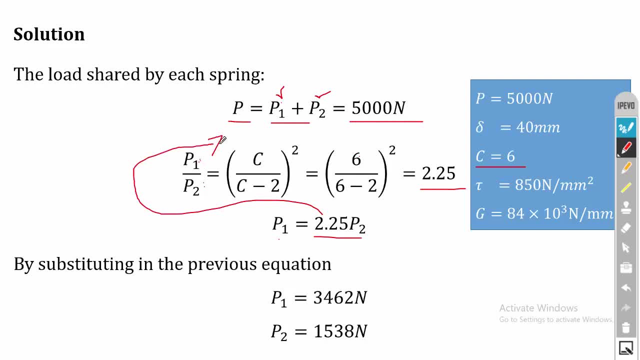 Now we can substitute this ratio in the first equation. Ok, In this equation we can substitute it. So by substituting the P1 value in this equation we will get 3.25 P2 and by solving it we will get P1 value as 3462 Newton and P2 value as 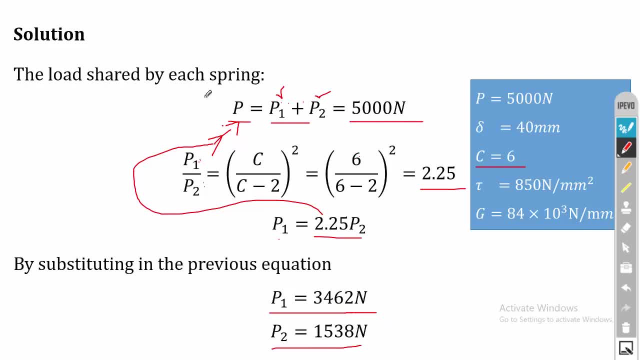 1538, Newton. So remember these two relations. So one is P is equal to P1 plus P2, and the second one is P1 by P2 is equal to C divided by C-2, the whole square. So calculate the relation first. 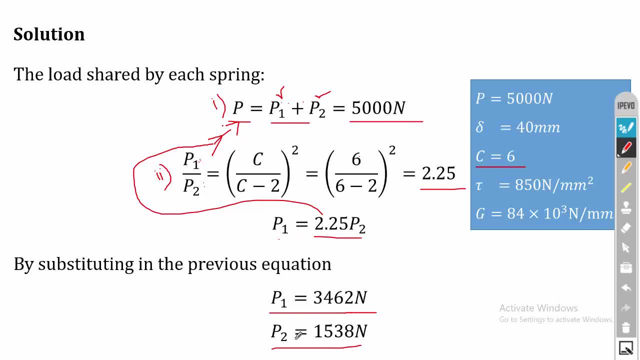 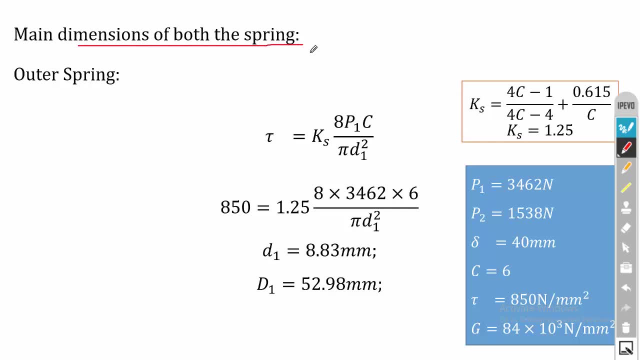 Then substitute the relation in the first equation and calculate the value of P1 and P2.. Now the second one is the main dimensions of both the springs. So we have calculated the value of P1 and P2.. Now we can split the design procedure into two, that is, design of. 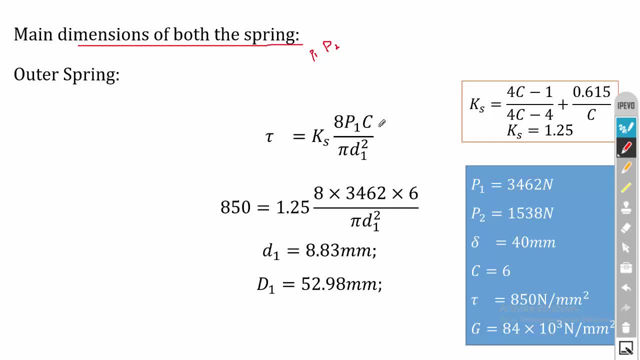 outer spring and another one is design of inner spring. So the main dimensions of both the springs: First I have considered the outer spring, that is, tau is equal to 8 Ks. I mean Ks8P1 because I have considered the outer spring C divided by Pi D1, square the diameter. 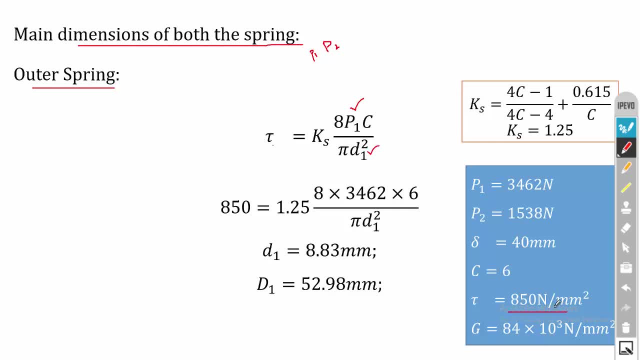 of the outer spring. So tau is given as 8.5 in the problem. we can substitute it and Cs. so Cs is well stress concentration factor and by substituting the value of Cs6 we can calculate the Ks value as 1.25.. So Ks is equal to 1.25. you can substitute that. Then P1 we 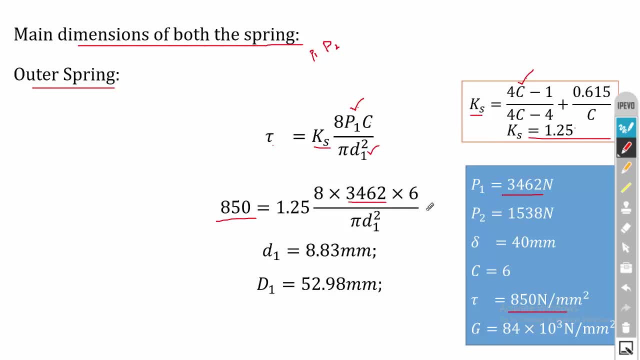 have calculated is 3462,. c is 6 divided by pi d1 square. So substitute all the data and calculate the value of small d1, that is 8.83 mm. Then we know that c is equal to capital D1 by small d1 in the case of outer diameter. 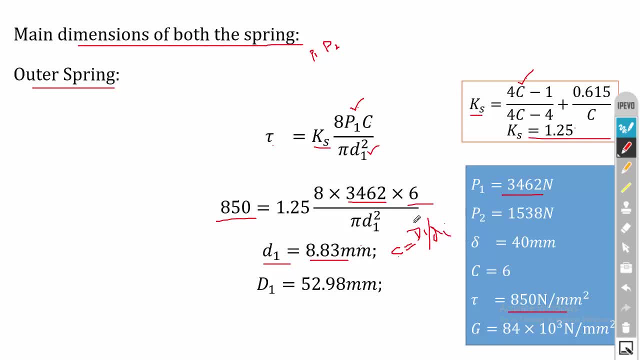 So use this relation. we know the value of c and d1 and calculate the capital D, that is coil diameter. that is equal to 52.98 mm. So now we have calculated the diameter for outer spring, then the next one is inner spring. 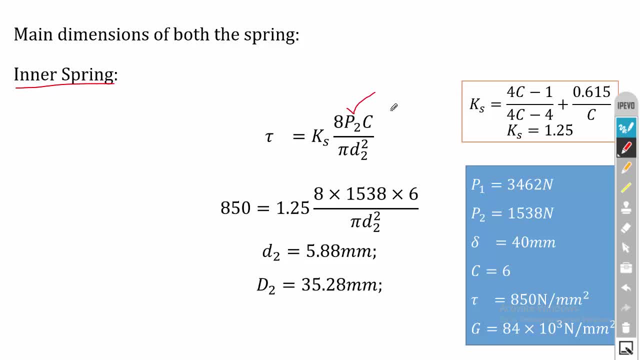 So here, in the place of p1, we have to use the p2 value, because we are going to consider the inner spring. So remember that two springs are there. one is outer spring and another one is inner spring. So outer spring is 1 and the inner spring is 2.. 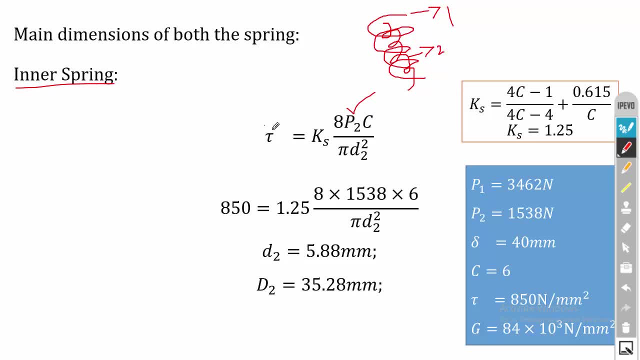 So 8.98 mm p2c divided by pi d2 square. so tau, ks and c values are common. So substitute it and substitute the value of p2 as 1538.. So that you will get d2 is equal to 5.88 mm and capital D is equal to 35.28.. 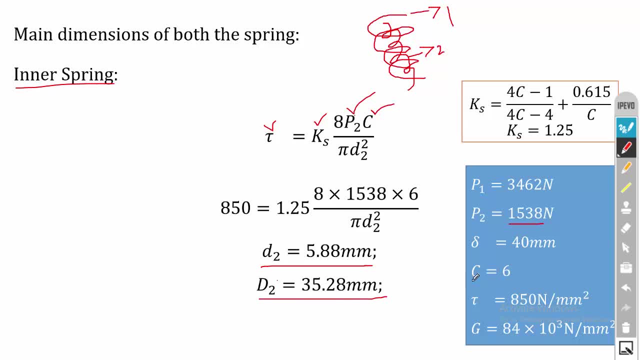 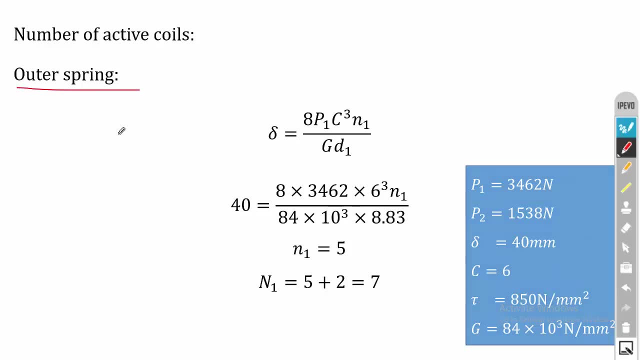 We can calculate the capital D2 by using the c relation. Now we have calculated the main dimensions. The next one is number of active coils. So first consider the outer spring. So it is like design of helical compression spring, but only thing, we have to split this. 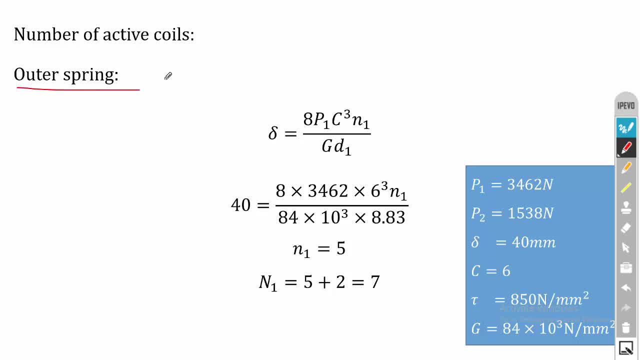 into two: outer spring and inner spring. So first consider the outer spring. that is, del is equal to- we know this equation for calculating number of turns: 8, p1, because it is outer spring. c cube divided by n1, divided by gd1, since we are considering the outer spring, 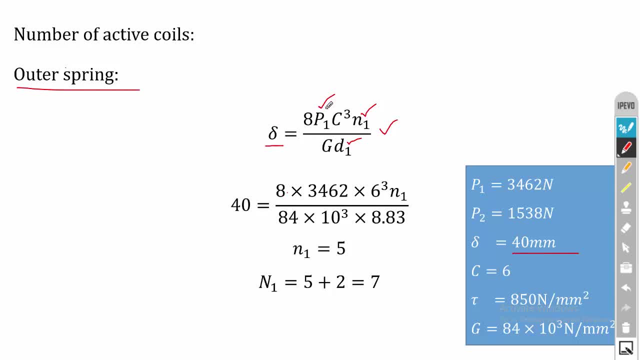 So del is given as 40. So I have to substitute the value of outer spring, So del is given as 40. So I have to substitute the value of outer spring, So del is given as 40. So we have obtained the value of outer spring. 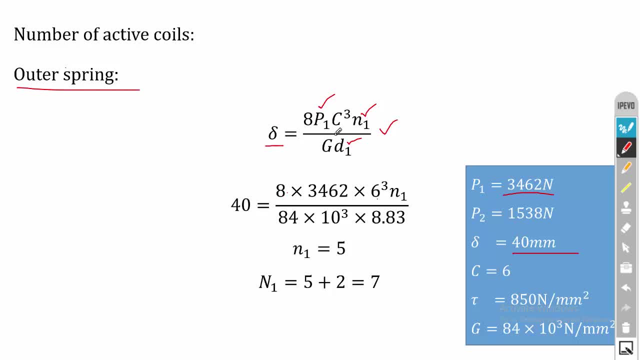 So I have to substitute with value of inner side, And this will be fニ n awareness power, which is f…"6, who is equal to 5, provided only D. So del is given as 50.. So total of total part time is 8, which is C. then del is given as 60.. 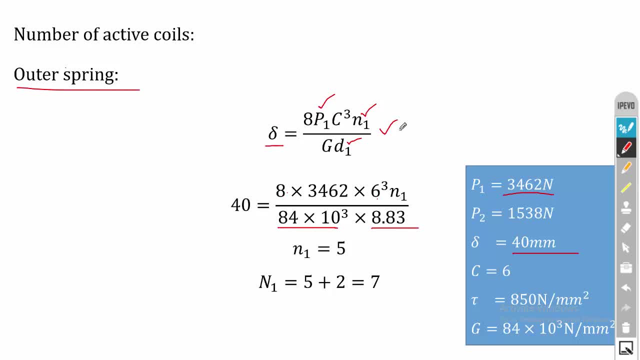 So this we calculate below in leads to exczzle this value of outer side, which is 68. So 2U1 is equal to 4.. So by solving this equation you will get small. n1 is equal to 5 and we can assume the ends. 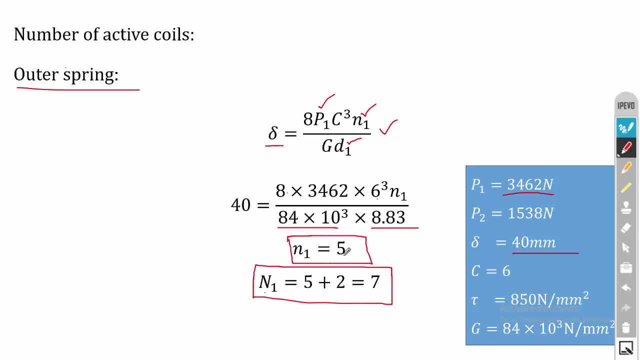 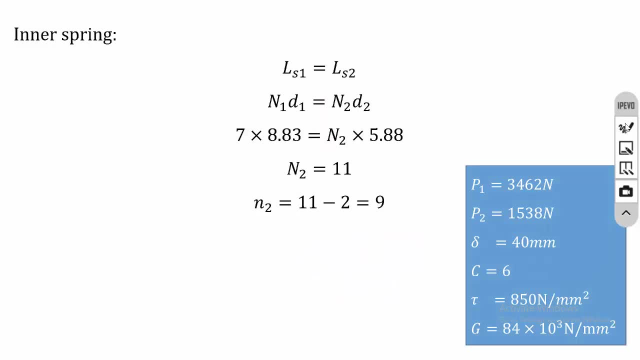 are squared and grounded So that N1 is equal to n1 plus 2, that is 5 plus 2, that is equal to 7.. Now the important thing is capital letters. You can write here you are showing that 4N1 plus 2 developer's four largest in the world. 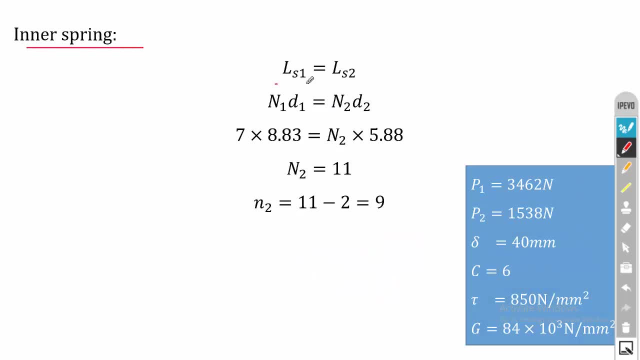 In the concentric spring the solid length is same. So by equating the solid length of both the springs we can calculate the number of turns of the second spring. We know that Ls1 is equal to Ls2 and we know that the solid length is N into D. 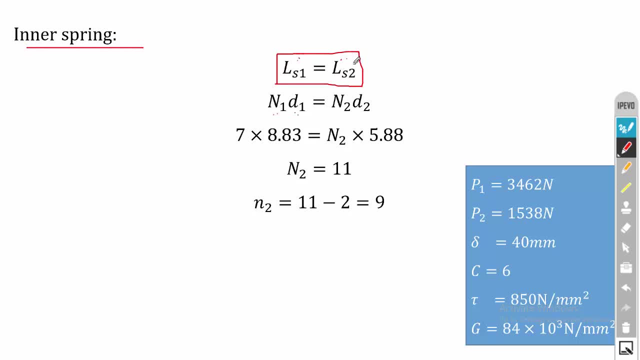 So in the case of Ls1, it is N1D, In the case of Ls2, it is N2D, And previously we have calculated the value of N1, D1 and D2.. So the only unknown value is N2.. 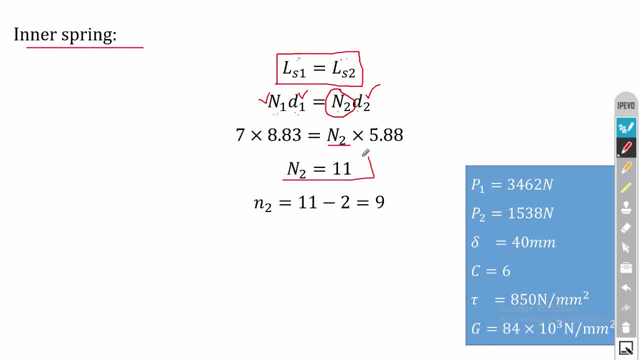 So substitute the remaining values and calculate the N2.. That is total number of turns for the inner spring. So to find the active coil, we will put: N is equal to N plus 2.. And if you want small n, then small n is equal to N minus 2.. 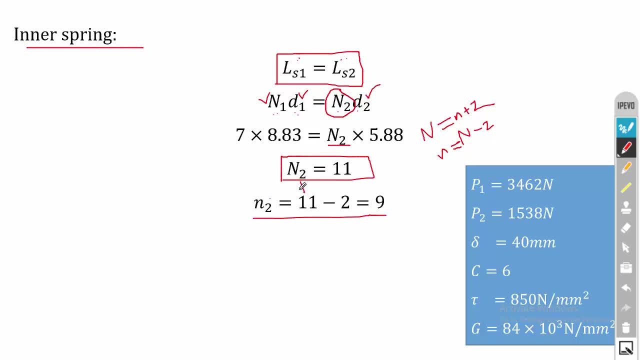 That is why I have substituted it here. N2 is equal to N2 minus 2.. That is 11 minus 2.. That is equal to 9.. So this is how we have to calculate the number of turns for the inner spring. 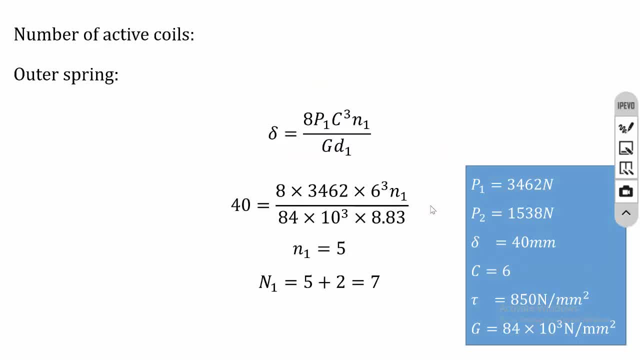 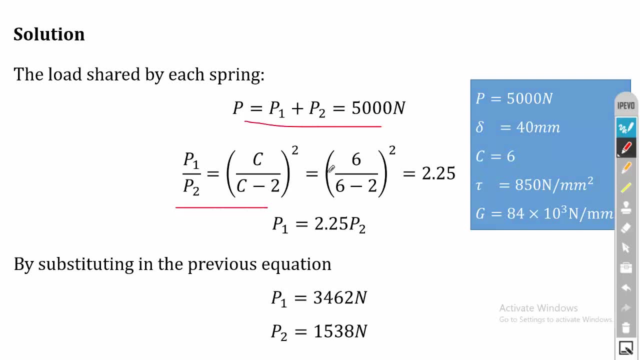 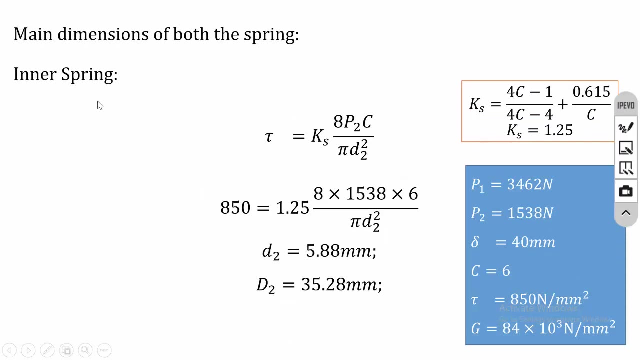 Remember that first we have to start from the load. use the two relations to find the load value, That is, P1 plus P2 and C by C minus 2, the whole square. Then split the design procedure into two. First calculate the dimension for outer spring, then inner spring. 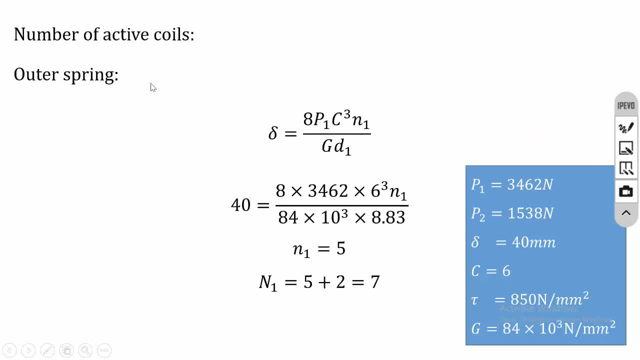 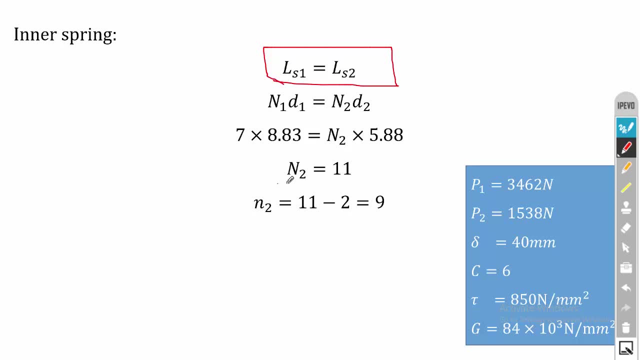 Then, for active number of turns, calculate the number of turns for active- I mean outer spring- Then, by equating the solid length of both the springs, calculate the number of turns for inner spring. So for inner spring don't calculate the number of springs by using the common formula. 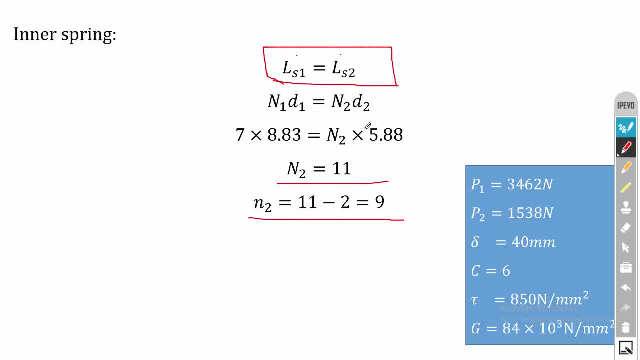 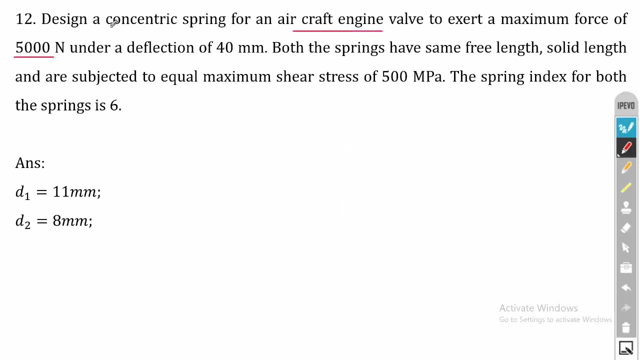 So we have to equate the solid length. That is very important. This is a critical point you should consider. So the tutorial problem is: design a concentric spring for an aircraft engine valve to exert a maximum force of 5.3.. 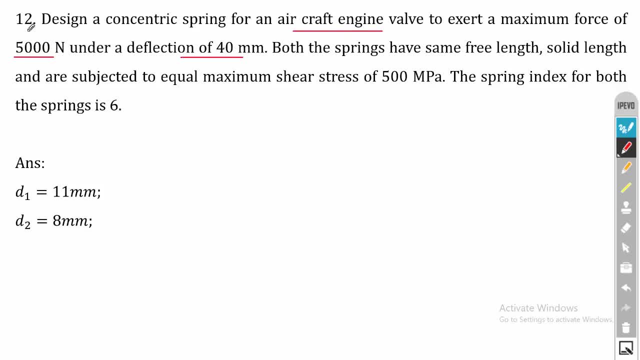 That is 5,000 N under a deflection of 40 mm. So the capital P value is 5,000 N and the deflection del is 40 mm. Both the springs have same free length, that is Lf, and same solid length. 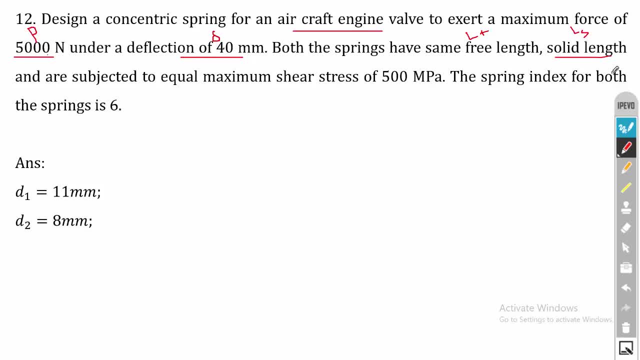 So Ls1 is equal to Ls2.. This statement will be useful for calculating the number of turns of the inner spring. And subjected to a equal maximum shear stress of 500 MPa. So tau is common for both. So tau is common for both the springs and it is 500 MPa. 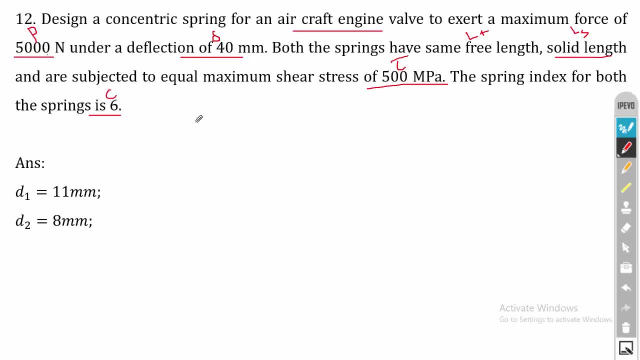 The spring index for both the springs is 6.. So c is equal to 6.. So we have to design the spring. So design the spring means initially you have to start from calculation of P1 and P2. Because once, if you calculate the P1 and P2, then you can start the design procedure. 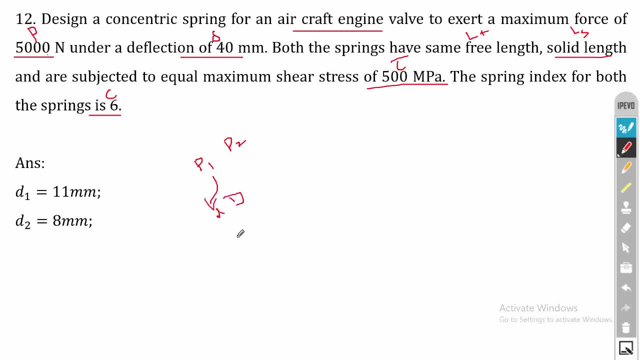 Then you have to calculate d, d, N, N, then finally L, F and pitch For outer spring and for inner spring. So the calculation of Lf and P is same as that of the normal compression spring, That is, Lf is equal to N into d plus 1.15 del.